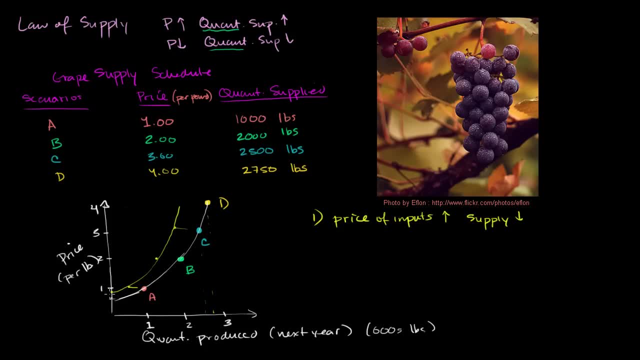 would also go up when you shift the curve to the left, because now all of a sudden it costs me more to produce even that first unit. And likewise if my price of my inputs went down now all of a sudden at any given price point. 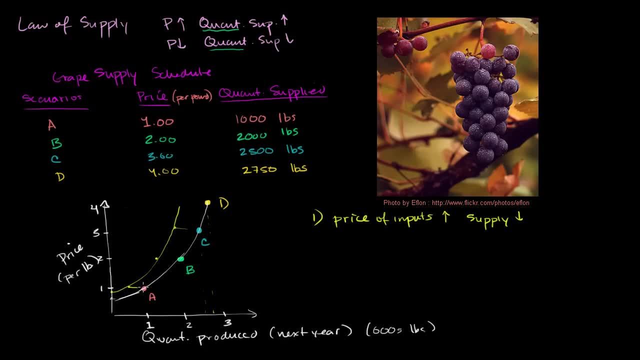 producing grapes would become more profitable And I would have more incentive to maybe produce grapes, OK. OK, So I would have to use grapes relative to other things and use more land for grapes than other things, And then you would have the whole curve shift to the right. 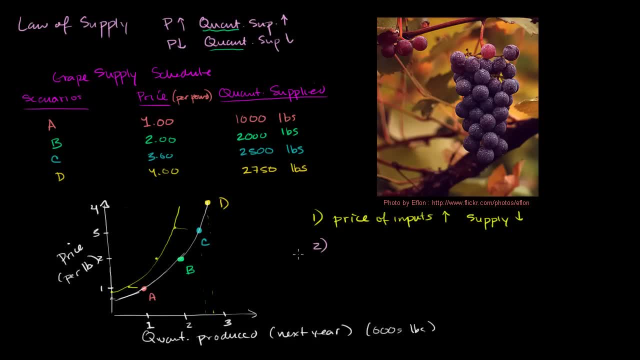 Now let's think about related goods. So what happens with the price of related goods? And when we think about this, we don't want to think of it from a demand point of view, because we're talking about supply. You want to think about it from the producer's point of view. 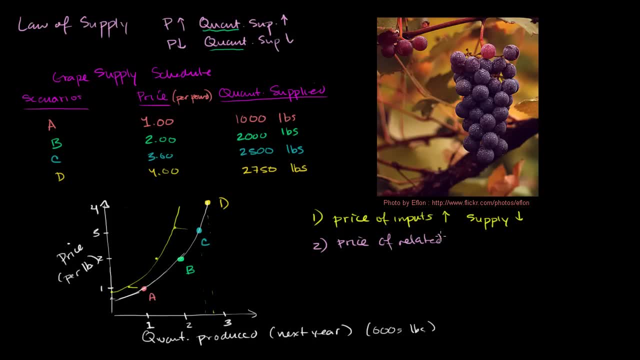 So when we think about related goods here, we want to think about substitutes for production. So maybe I'm a farmer and I know very little bit about farming, so I don't even know if this is possible, But maybe on my land I'm saying well, 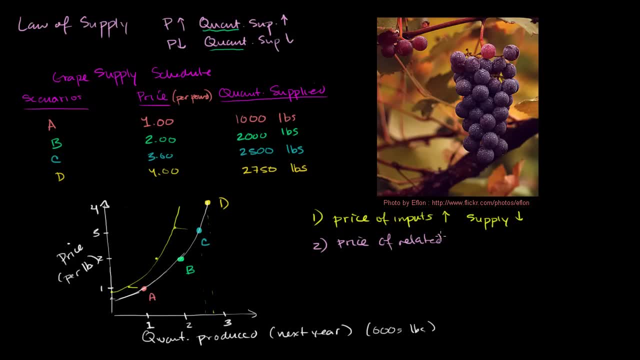 some of my land is going to be for grapes and some of it is going to be for blueberries, And so what would happen if the price of a related good, in particular blueberries, what would happen if the price of blueberries went up? 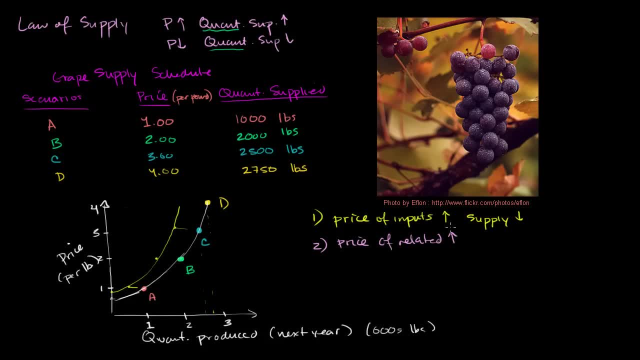 Well, if the price of blueberries went up, then I would say, wow, maybe I can do better with blueberries and I would allocate more of my land to blueberries than to grapes. And so, once again, if the price of related goods 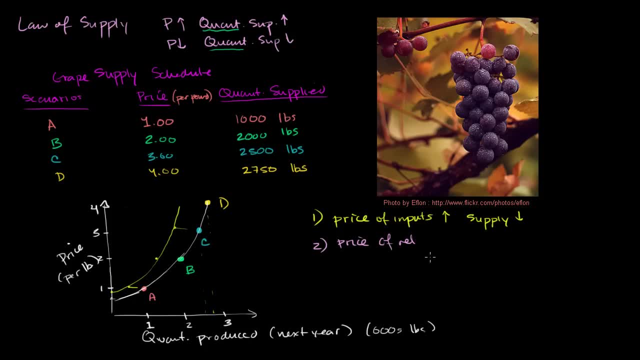 well, it depends which related goods. but if the price of productive substitutes, so price of other things I could produce, if the price of other things I can produce goes up, then my supply of grapes, once again my supply of grapes would go down. 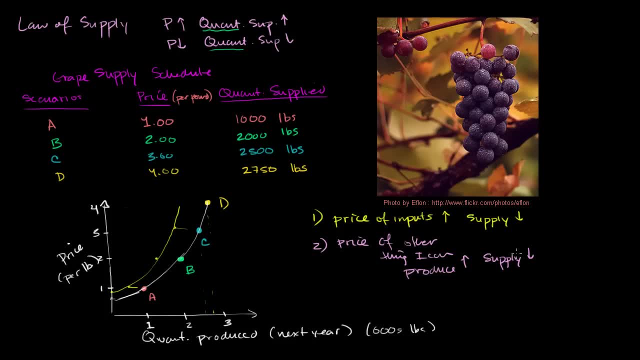 Now the important thing is, in any of these circumstances, literally just think it through. Do not just look at what I'm writing here and just try to memorize in some form way, shape or form. This is really just a way to think about things. 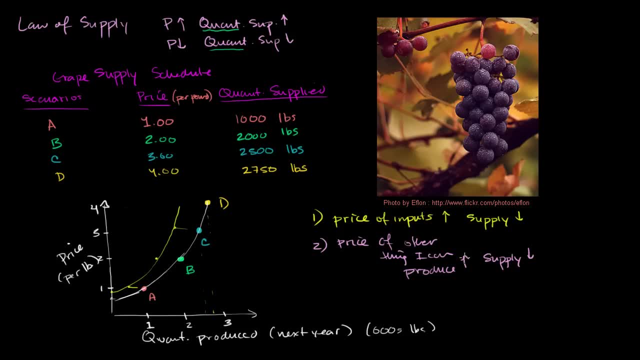 Hey, obviously, if I can make more money off of blueberries, now, all of a sudden, I'm going to allocate more of my land to blueberries than to grapes, Supply of grapes will go down. Now let's think about what happens. 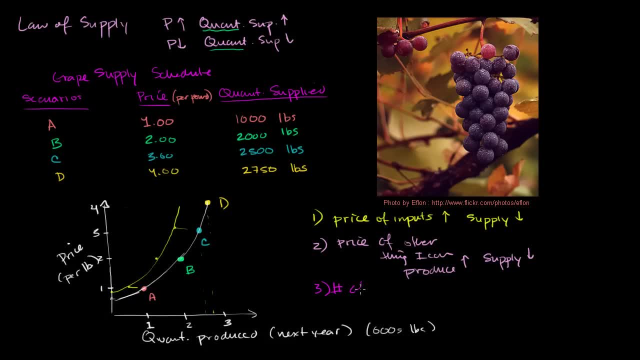 with the number of suppliers, And this one is pretty good. It's pretty common sense: The more people they are supplying, the higher the supply would be. So if the number of suppliers goes up- and now you wouldn't imagine this- 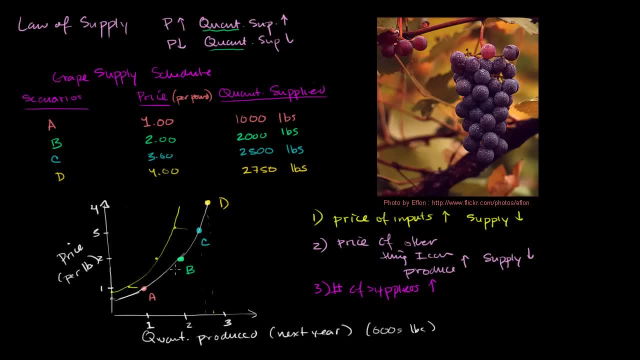 is a curve, maybe for the aggregate supply. So if the number of suppliers go up, then the aggregate supply would go up at any given price point. If the number of suppliers were to go down, then the aggregate supply would go down at any given price point. 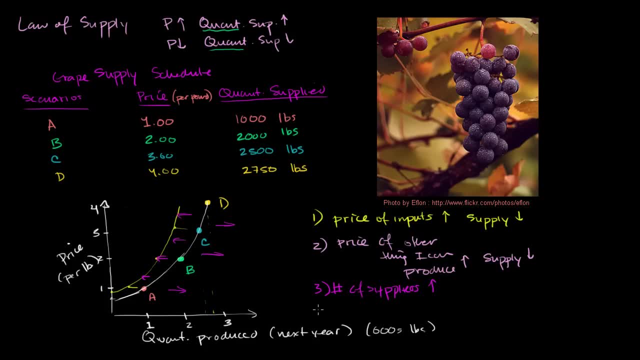 So this one, hopefully, is somewhat obvious. Then we could think about things like technology And so this is just: maybe there's some innovation, some new type of seed that with the same amount of work, the same amount of land can produce that many more grapes. 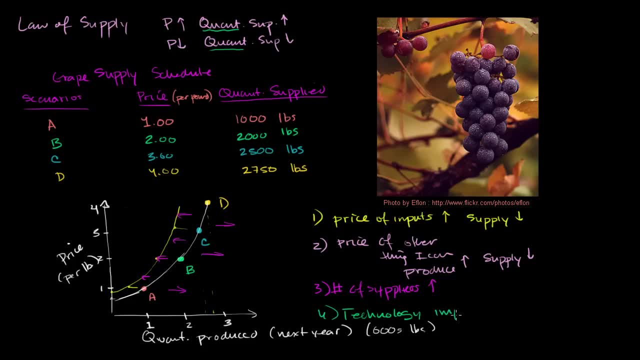 So if you have technological improvements- I'm assuming we're not going to go into some type of dark ages- If we have technological improvements, then that will also make the supply go up. You can also think of it as it might make it cheaper to produce. 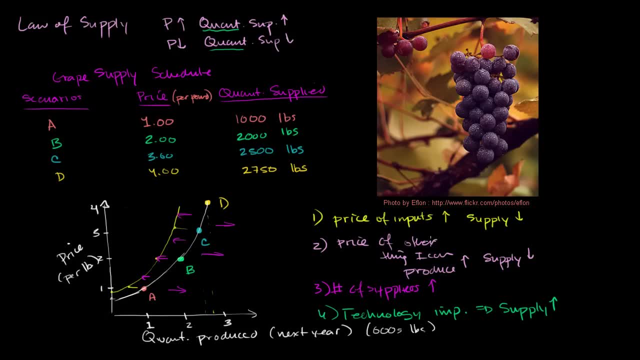 So it's kind of the same thing here. The price of inputs might go down, So that would make your supply go up. Or you could just say, hey look, there's just going to be more grapes popping off of these new types of vines that we got. 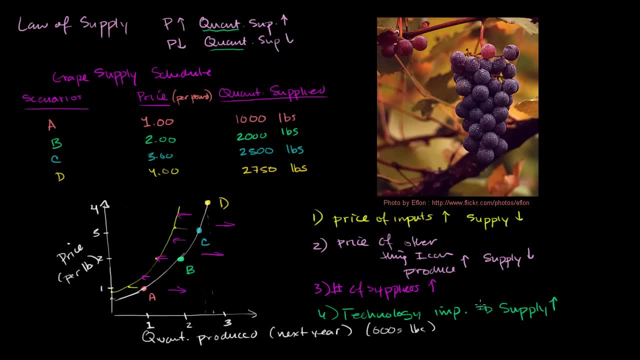 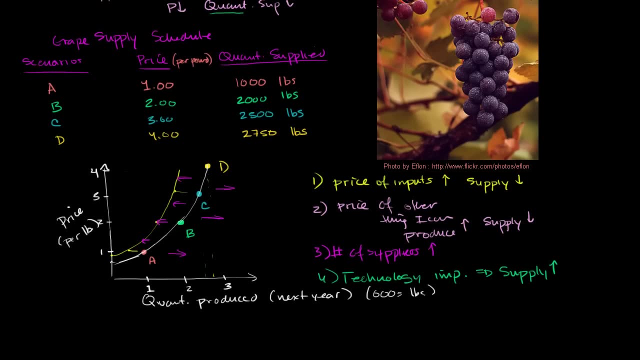 So we're just going to produce more grapes. And then the last one I'll cover- and it's a little bit strange in the grape analogy- is the expected future prices, Price expectations. And let's go away from the grapes, because grapes are perishable goods. 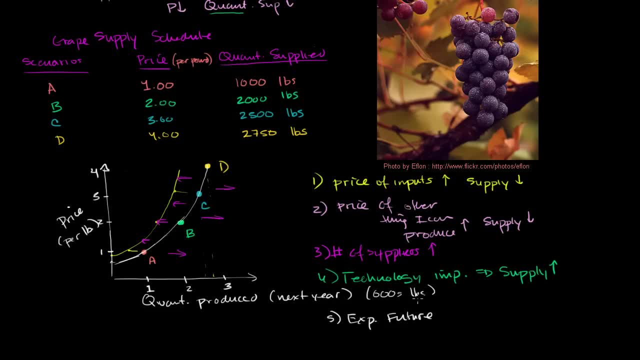 They go bad. It's not like you can save goods to use them later, But if, let's say, you are an oil producer and oil is something that you can store and you can use it later. if you expected oil prices to be neutral today and then tomorrow, all of a sudden, you are sure that oil prices are going to go up in the future. you're sure that a year from now, oil prices are just going to go through the roof. what's your incentive? Well, you should hoard all of your oil. 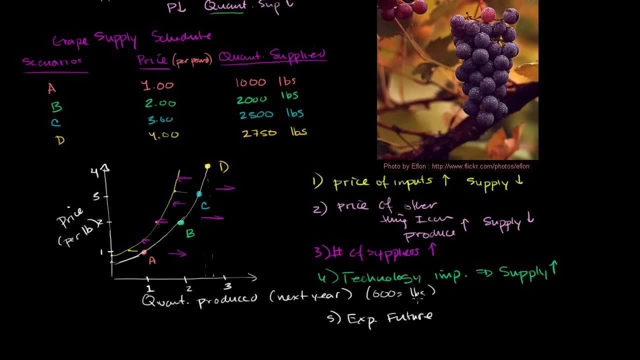 Do not sell it today and wait to sell it in the future if you're sure that's what's going to happen If there's a change in expected future prices. so if you go from neutral to expecting prices go up in the future, then you're going to hoard your goods.